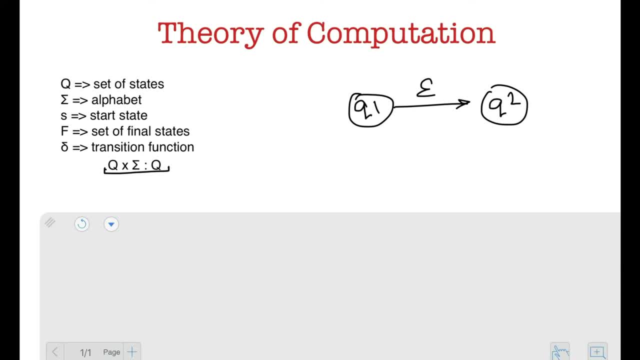 and my transition function right here does not account for that, because it says that it has to be from Q cross sigma to Q. So I can have something like: let's say I have a state Q1, let's say Q3, comma the alphabet 0 and this going to, let's say, Q4.. This is actually possible. 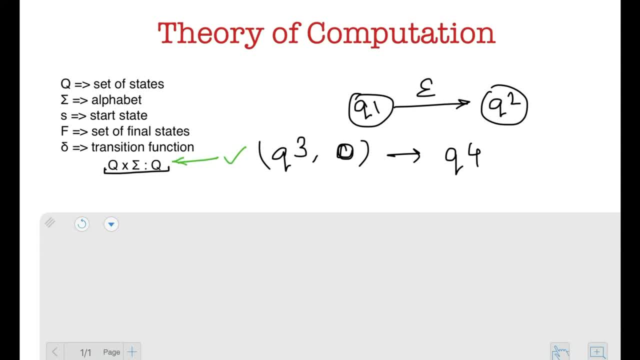 according to this definition that I have right here, but something like this, which is Q1 and epsilon going to Q2. This isn't allowed according to this definition because epsilon is not an alphabet. So it's actually very simple to account for: epsilon moves, The only 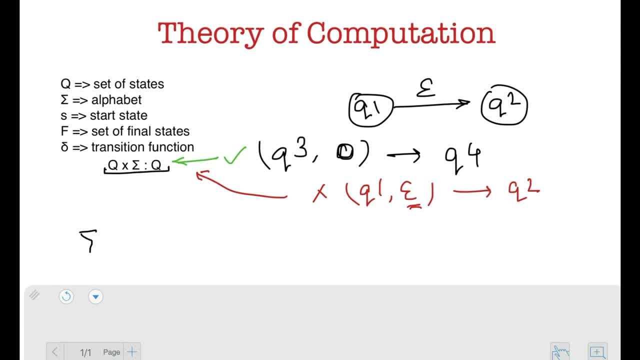 thing we have to do is we define delta as delta as being from Q cross sigma union, the set containing just epsilon to Q. So when I do this, then my this definition, this example right here, Q1 comma, epsilon going to Q2, actually fits, because I added the epsilon right here. So that's all we. 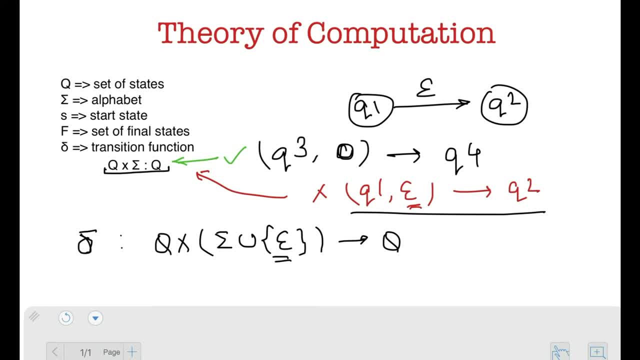 have to do if you want to account for epsilon moves. The second thing that we want to account for in non-deterministic automata are multiple transitions. So let me first just get rid of this right here. So, for our multiple transitions, what do I have? I have some Q3, which can go on a. 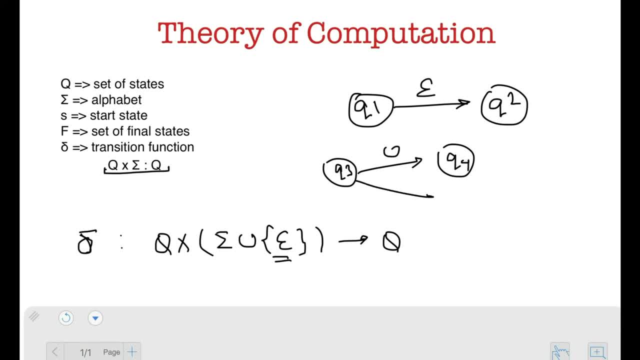 zero to Q4 and it can go on a zero itself to Q5 as well. So once again, this can't be accounted for because my transition function needs to give me one state, which is in the case right here, because if I take Q3 comma zero, then it will give me Q4 as well as Q5 and not just a single state. 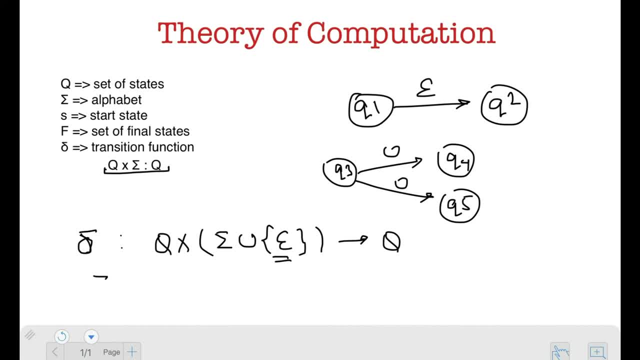 So to account for multiple transitions, what do we do? So let's say that it goes from Q cross sigma to the power set of Q. because when I say power set, what does it mean? It means that I am taking all subsets of Q. So if I say that Q delta goes from, 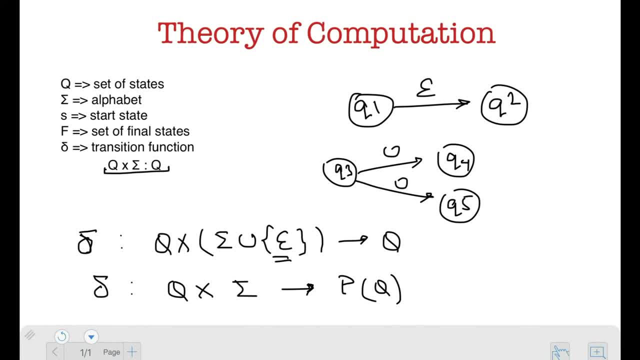 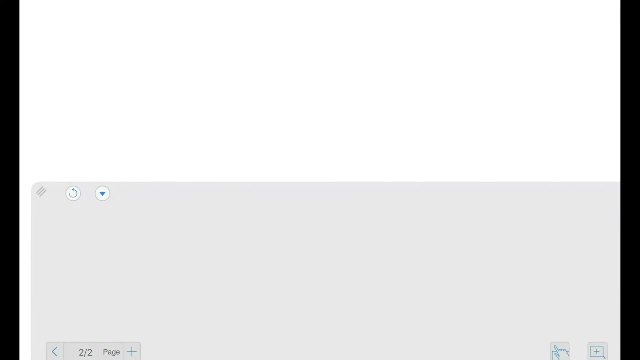 Q cross sigma to power set of Q. this power set of Q will definitely contain an element which is Q4 comma Q5.. So this actually accounts for my multiple transitions, this one right here, and if I want to give a more complete definition, now for my non-deterministic automata. the rest of the things remain the same. My Q is my set of. 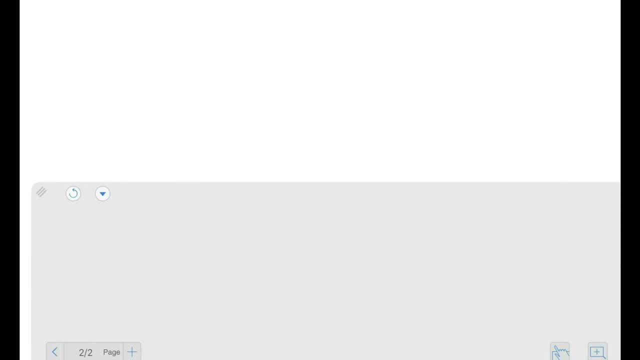 states. sigma is my alphabet, S is my start, state F is my set of final states. The only thing that changes is my delta is now from Q cross sigma. Now let's say that I have a set of elements and I have a set of elements and I have a set of elements. 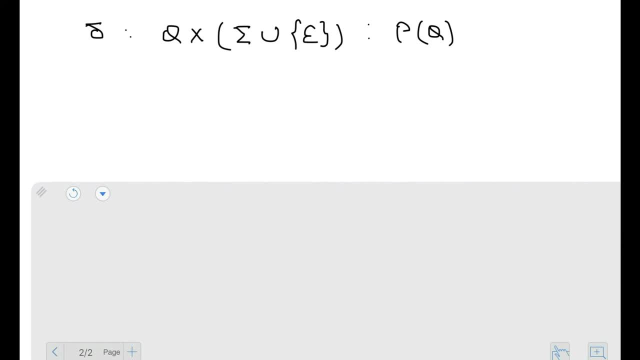 and I have a set of elements. I need to define a non-deterministic automaton, and one thing that I want to talk about at this point is the start state in non-deterministic automaton automata. sometimes we also say that it can be a set of start states, although we can always have 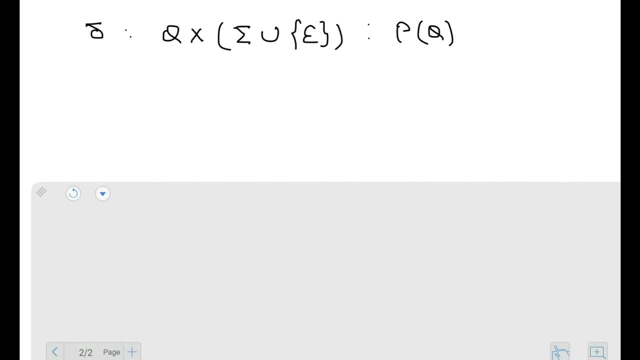 automata with a single start state, and that's what we are usually going to do. but in theory it is possible to have multiple start states in a non-deterministic automata automaton. so that's another thing that we do change sometimes. so we represent it with a capital s and we say: 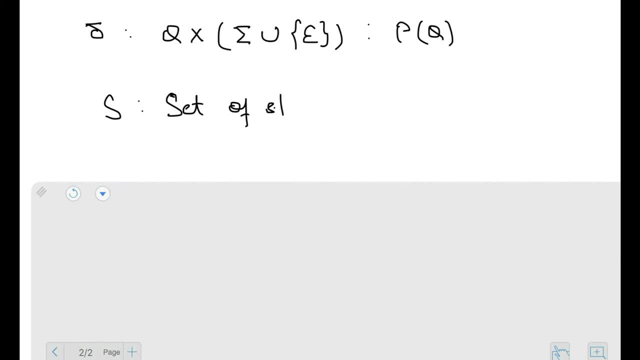 that this is my set of start states, start states, and we can always change this to epsilon moves. so let's say, this is my start state right here, which is q0, and i have an epsilon move to q1. i have an epsilon move to q2. this, some people might say, is the same as having start state q0. 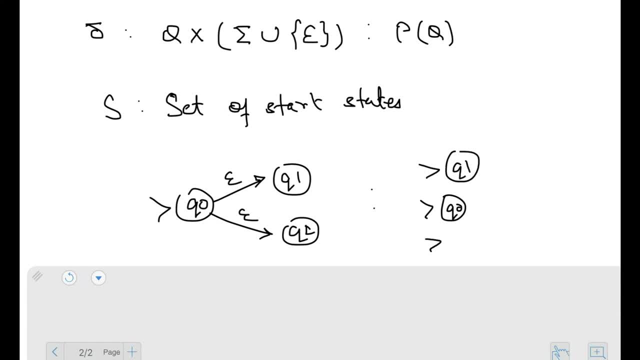 start state Q1 and start state Q2 and then continuing my automaton right here. so this is also valid. we could say that S can be a set of start states in non-deterministic automata, so this isn't wrong, but we'll just stick to a single.